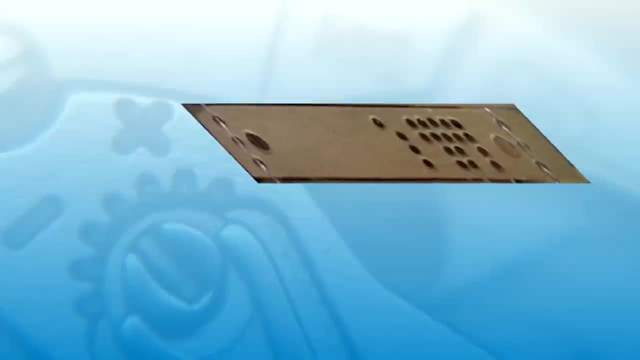 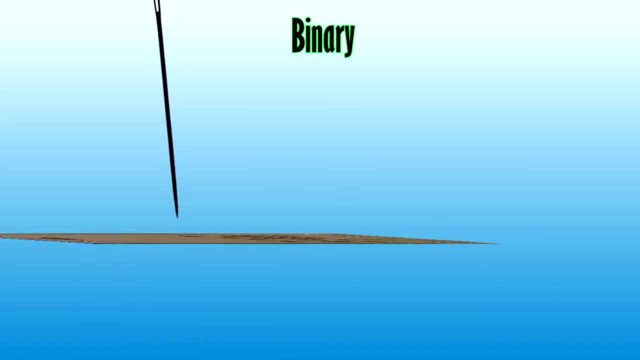 stored on cards with holes, And there was a mechanism that would go along the card and try to push a pin through, And so either the pin would go through or it wouldn't. It's binary, It's: either it does or it doesn't. 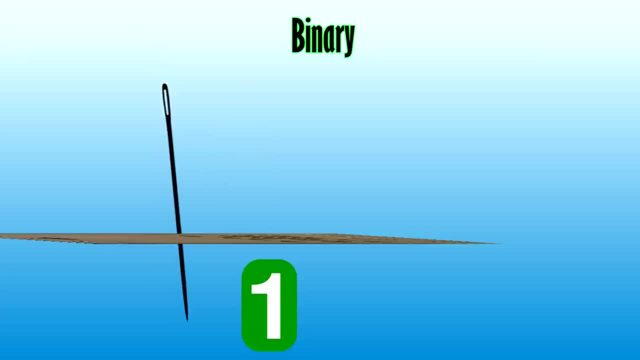 It's a one or it's a zero, And so if the pin goes through the hole, it would allow a rod attached to it to lift, which lifts the string and lifts the associated thread. And if the pin does not go through a hole, the pin doesn't move and the thread doesn't. 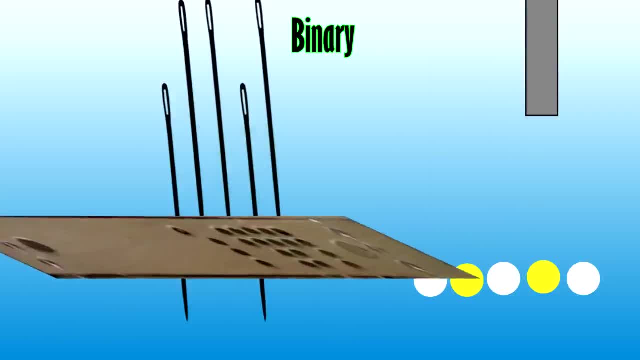 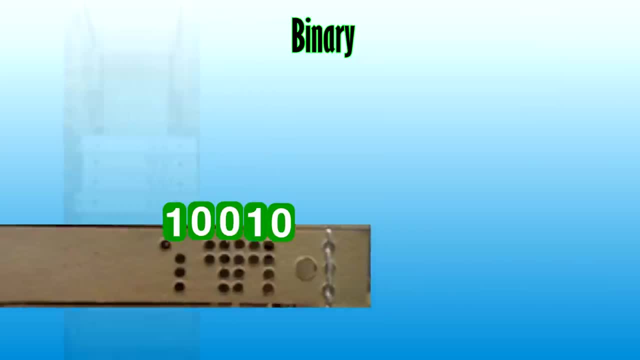 move. So, essentially, the card would hold a preset pattern that is read by the loom And serves as a guide, giving the direction to the threads, one at a time, And with this contraption you could create very fancy pieces of weaving. 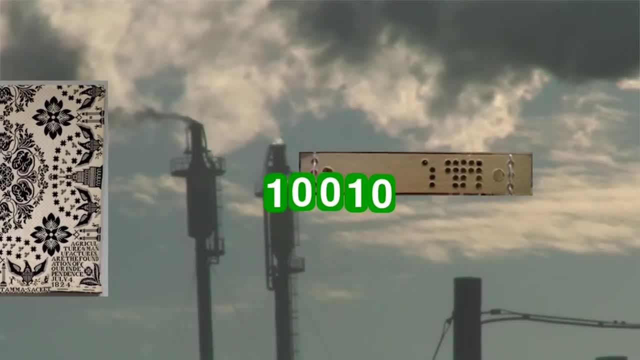 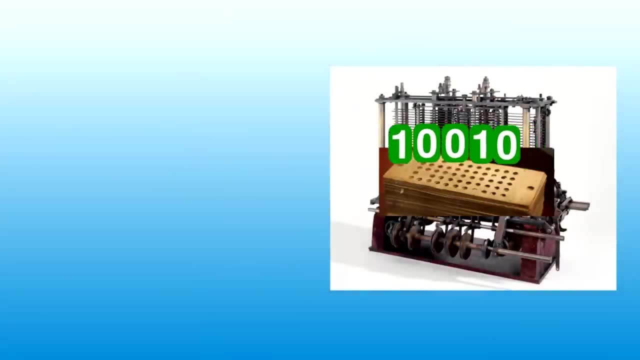 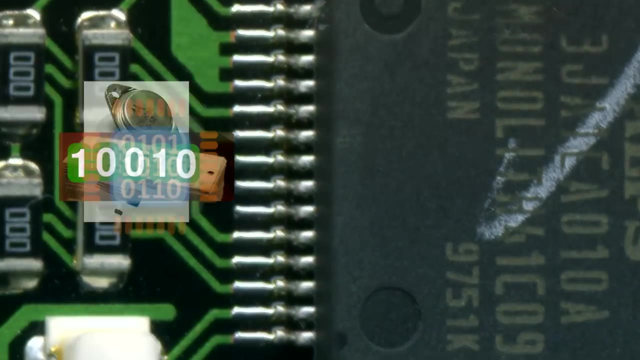 And this idea of there being recorded information read by a machine was quickly borrowed to be applied to mathematical computation. Charles Babbage invented the analytical engine in 1837, and it was basically a calculating machine. Eventually, transistors are invented, which replace punch cards as a way of transferring. 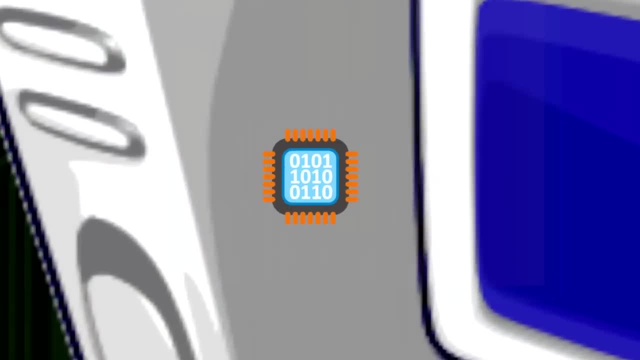 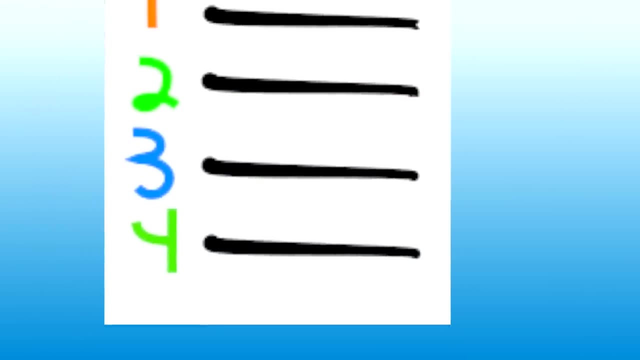 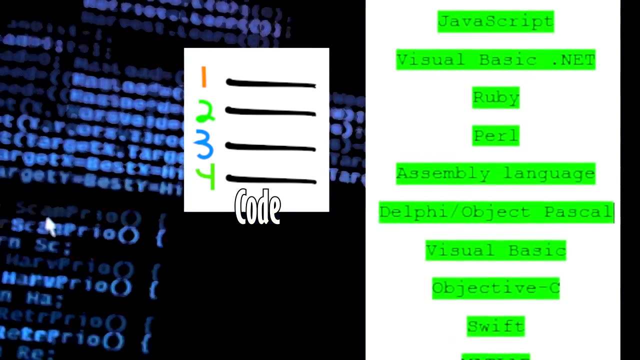 data. Nowadays, we use computers that have billions and billions of transistors, but still carrying that same basic idea of on and off to carry data. As a way of harnessing these various combinations of transistors, we use code. Computer programmers use different languages, whether it's Python for gaming, Java for 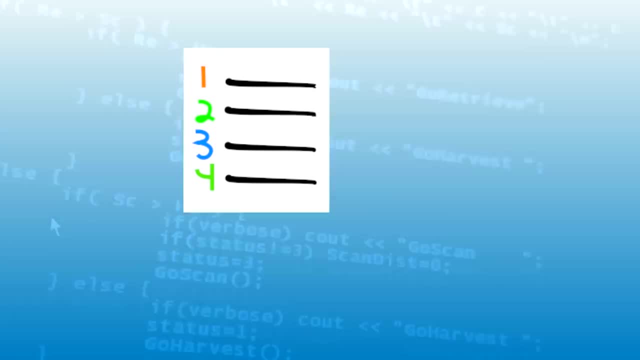 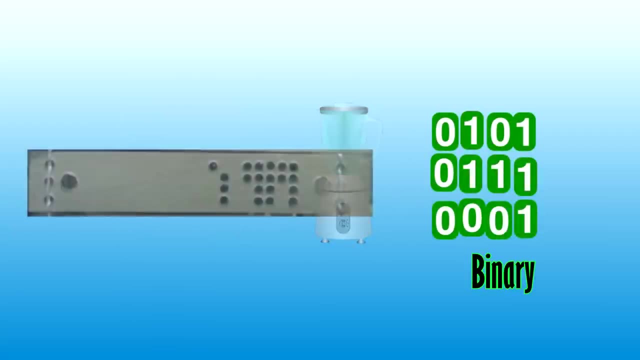 desktop applications or Objective-C for an iPhone app. A computer program is only a text file, following those rules, and it's eventually translated into something the computer can understand, just like the pins on Jacquard's loom. a computer can only understand two things. 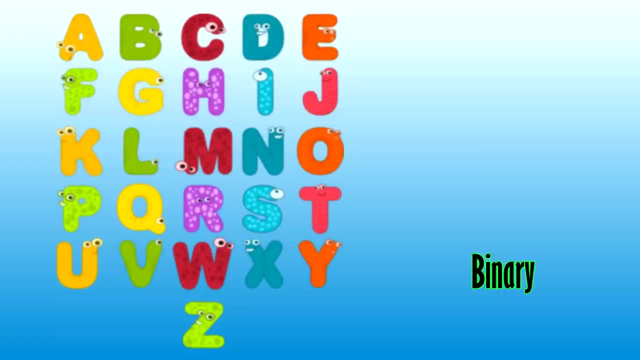 Think of 1 and 0 as the alphabet of a computer. It's like if you look at the alphabet of the English language: there's only 26 letters and by themselves they're meaningless, But when you combine them into different ways, you get the Great Gatsby or Romeo and Juliet. 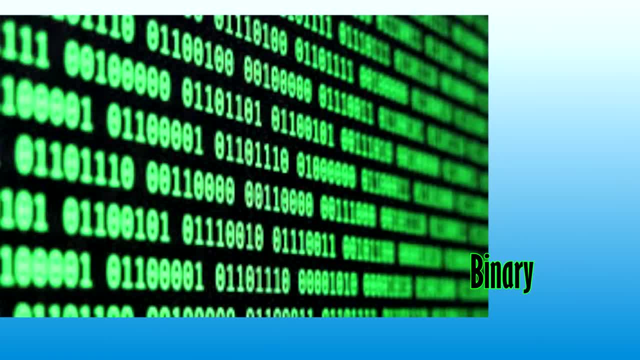 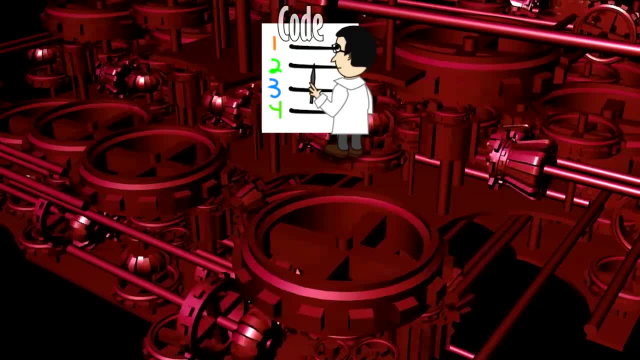 In the same way, billions of different combinations of 1s and 0s have the potential to give us Microsoft Word or iTunes, And the process goes like this: in the top level, you have a human writing code for a specific computer language. 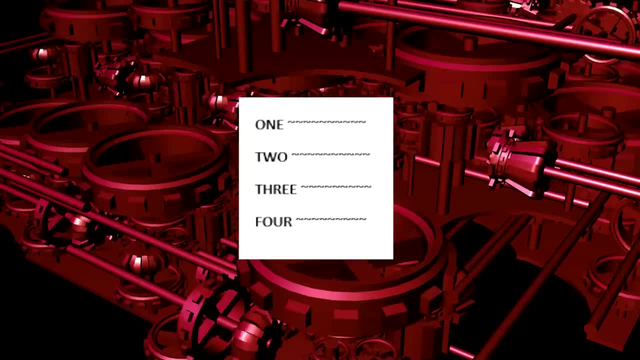 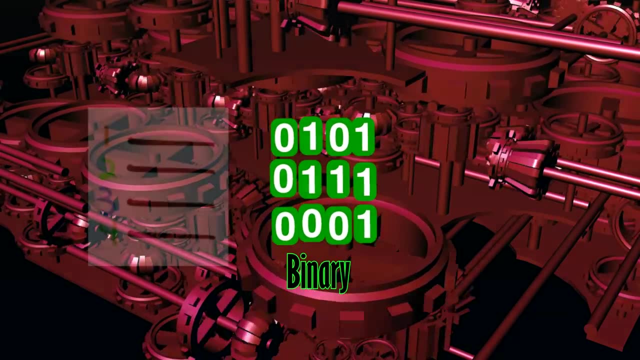 And after this the code is translated or compiled, And finally the code is translated into binary or machine language by an assembler. So because we have a way of translating human orders in the form of code into 1s and 0s.